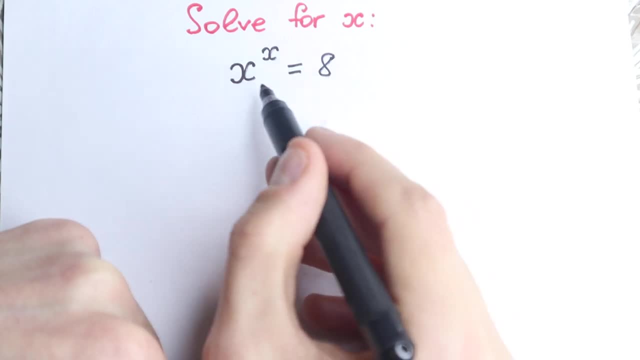 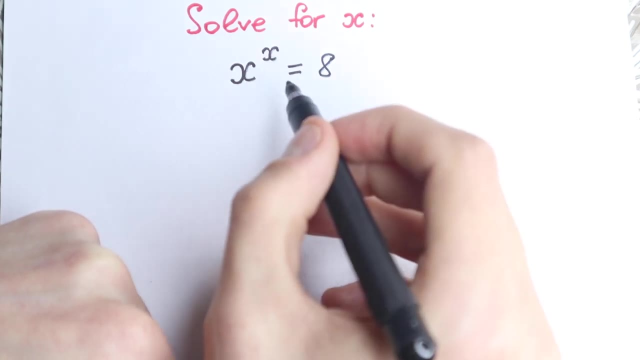 we cannot simplify this more or write it in another way, but this x to the power, x, it's really great to to write it in another way, to simply not like simplify or express this in another way. First of all, we have our x in our power. this is like a difficult part because 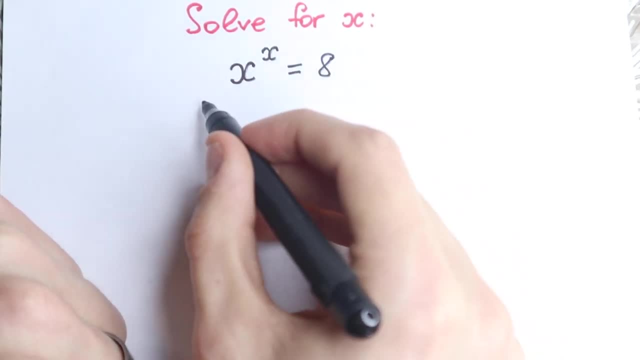 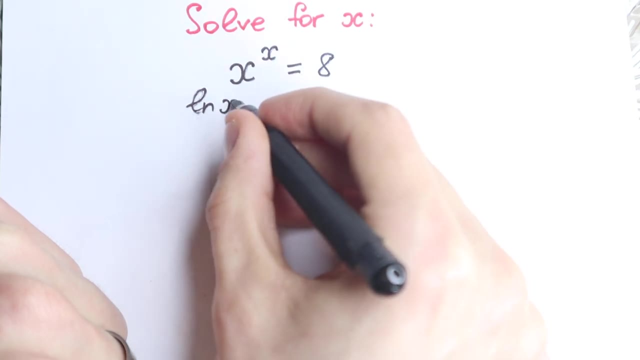 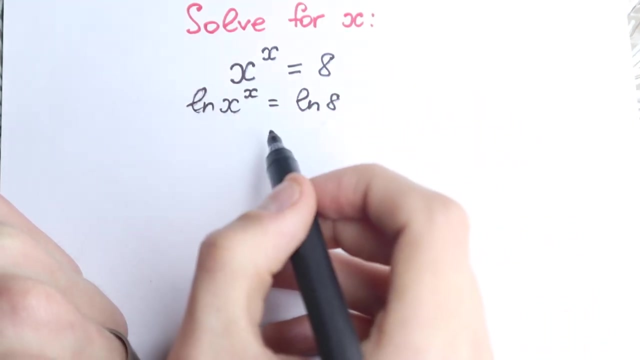 it's not good to have x in a power, so we need to apply natural log on both sides. okay, Let's do this, so we have natural log. yeah, my marker doesn't write so: natural log x to the power, x equal to natural log 8.. So what I did? I just apply natural log on both sides and students. 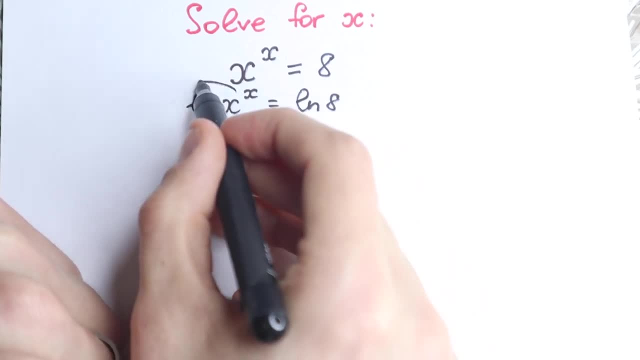 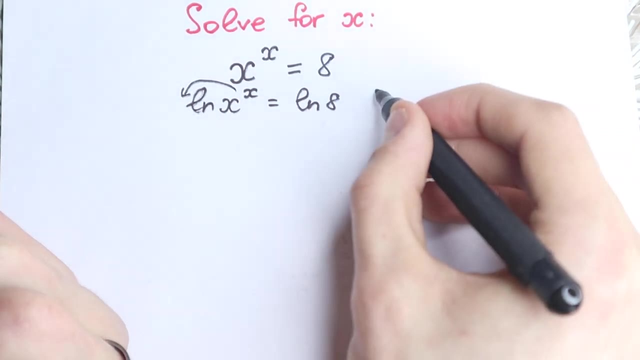 ask me for what I do that. for what? Of course I do this because this x needs to jump right here, because this is the main log property and let's do this right here. so of course I can write this rule. so this is our natural log. for example, a to the power b, this is equal to b times natural log. 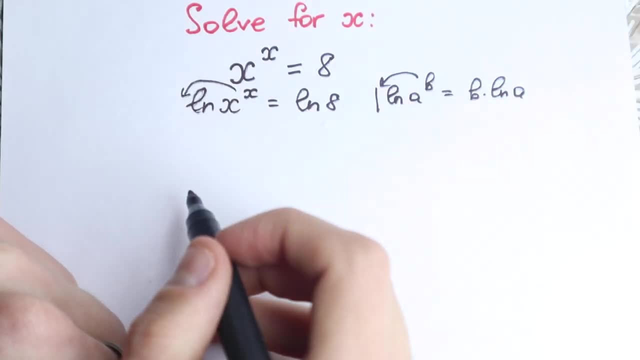 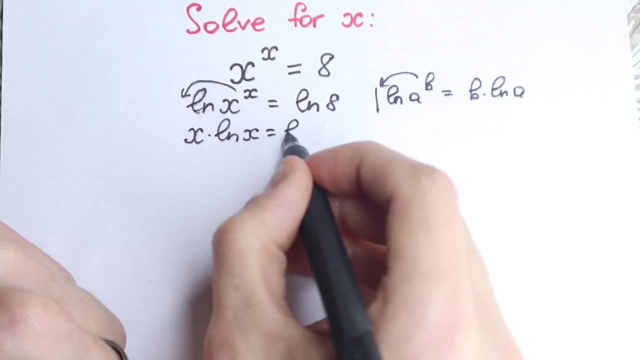 so this is the main log property. okay, So x jump right here. as a result, we have x times natural log, x equal to natural log a, 8. And a lot of students say that, okay, right now we have like a more complicated expression. so right here we have a better expression for us. right here we. 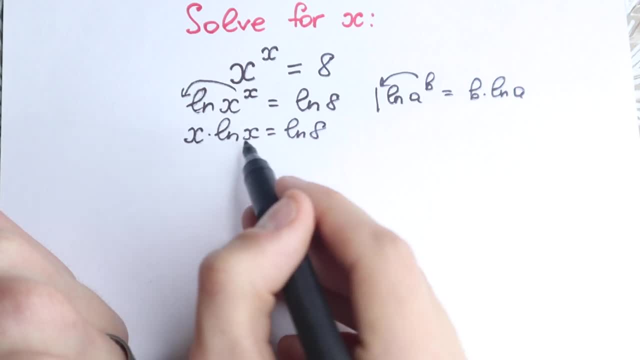 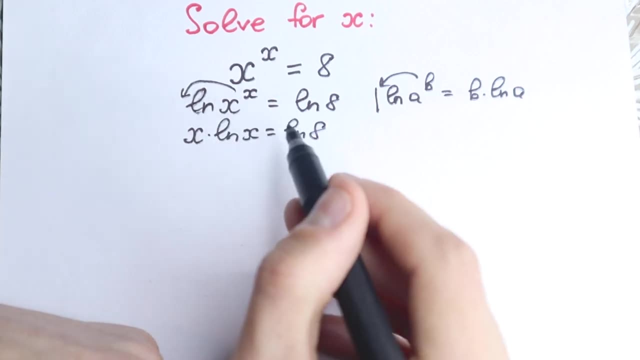 have a more complicated. we have natural log. we have, we have a product. we have natural log on the right hand side as well. so a lot of students don't know why I take natural log, why I apply natural log on both sides And then I want to show them the second trick. so it was our first trick and 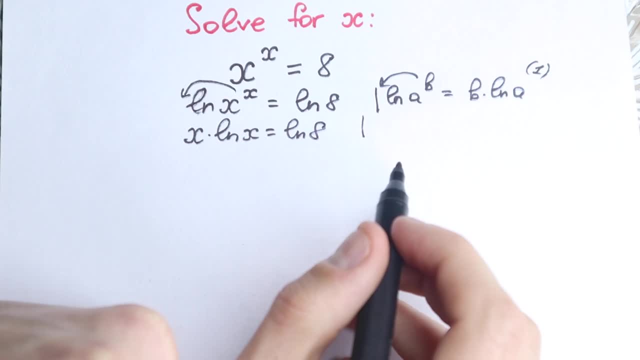 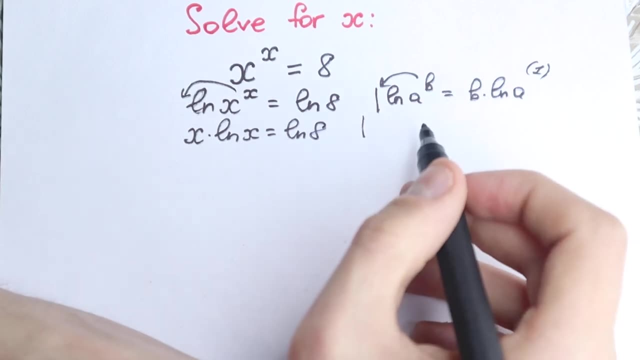 the second trick is not like a trick. I would say this is a great theorem, this is a great function, this function called Lambert W function. so a lot of students don't know about this function, want to learn or learn and don't understand or understand and learn this function. so I wanted 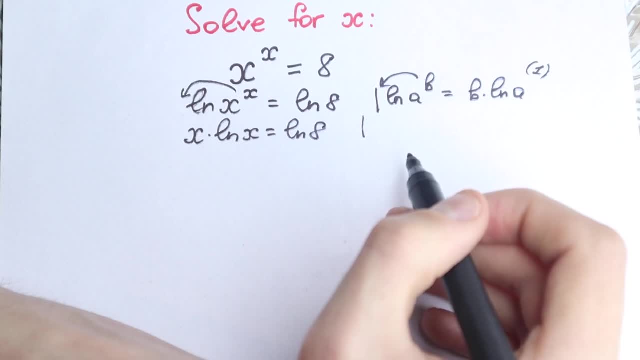 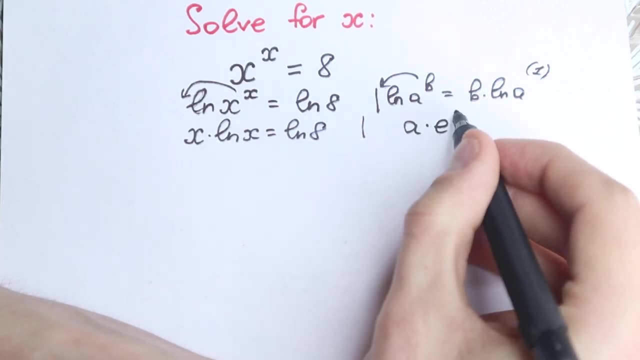 you to understand this function, and I'm going to explain this function in very simple words. try to you to understand. So, first of all, imagine that you have expression like that: a times e to the power, a. just imagine you have something like that, this expression where a is like wherever you want, expression doesn't matter. 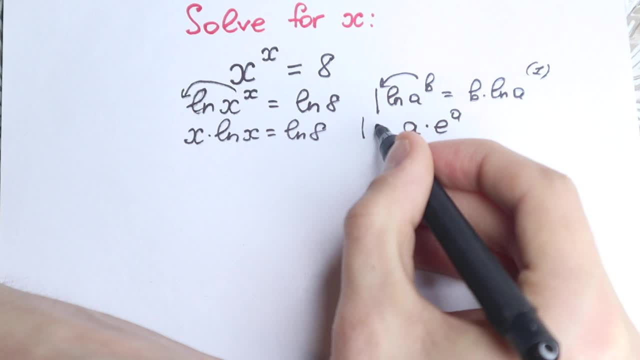 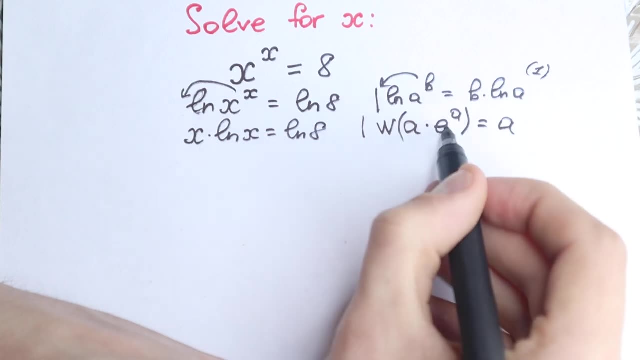 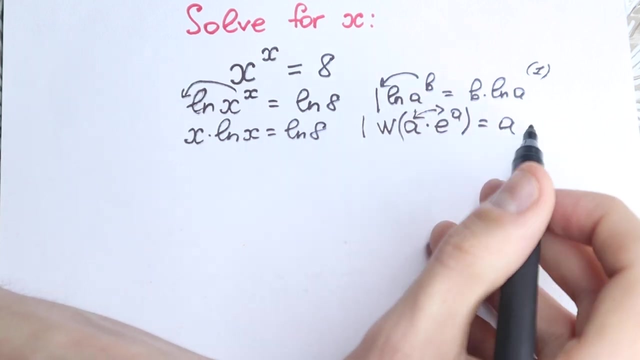 long short expression and if you apply Lambert W function from this expression, this is equal only to our a, so you need to have like a and a right here as a power of e, so this expression need to be the same. then you apply in Lambert W function and the result is our a. Let's look at our function. 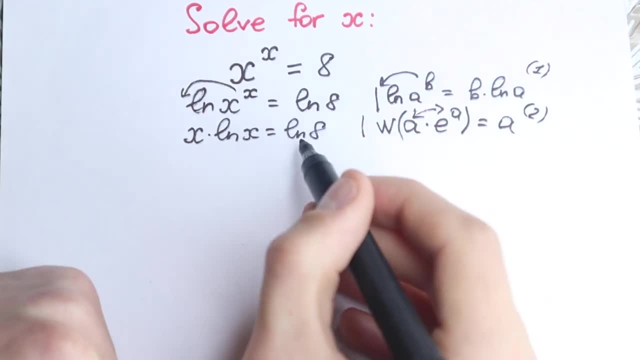 so this is our a. Let's look at our function. so this is our a. let's look at our function. this is second trick. let's look at our function. so we have natural log 8 on the right hand side. this is a constant, so we just need to leave the iterate here, because we cannot like express this in another. 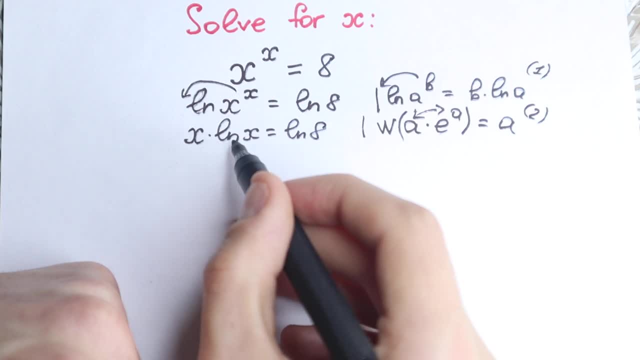 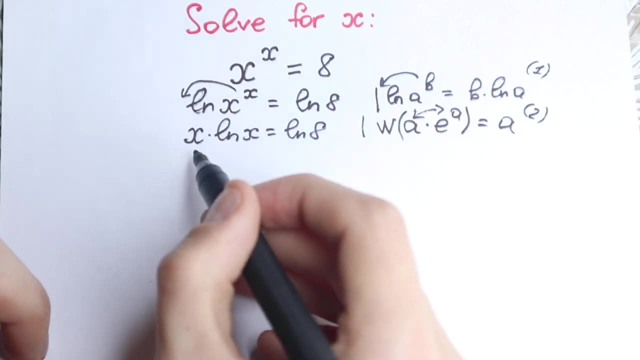 way. but on the left hand side we have x times natural log x. so we we wanna, we try to create something like that. first of all, we need to create e. let's look at it: we have x, we have natural log x. with natural log x it's a little bit harder to do this, but with x this is really great trick, because 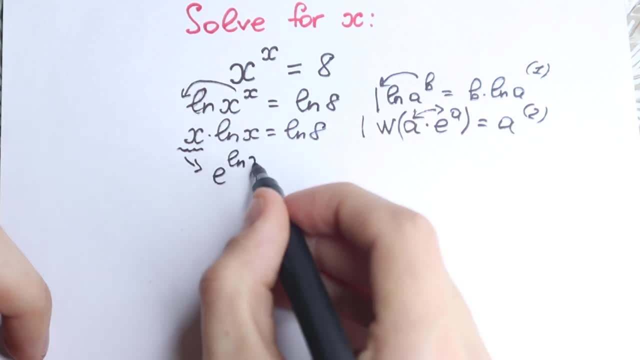 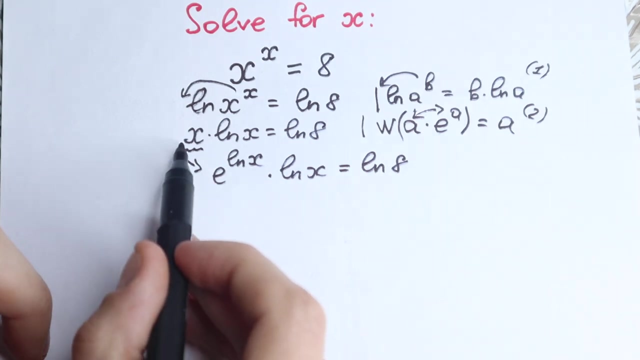 this x can be written as e to the power. natural log x. okay, and then times natural log x. this is like a from logger logarithm from your school: uh trick, yeah, and equal to natural log natural log 8. okay, what i did, i just write this: instead of this x, i write e to the power natural log x. 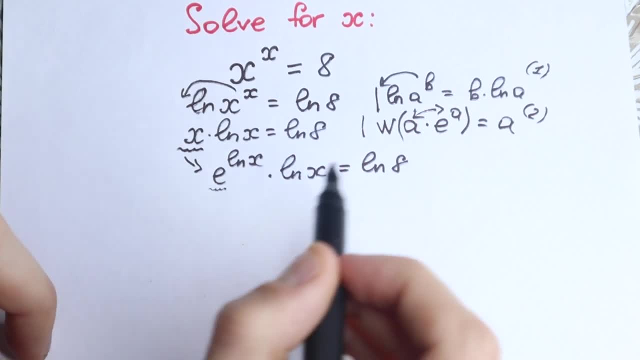 okay, right now we can easily find this e. we have this e. right here, we have this e and if we look closely, this natural look x, for example. we make a substitution. this is our a in our, in our heads, yeah, only in our heads, yeah, and this is the. 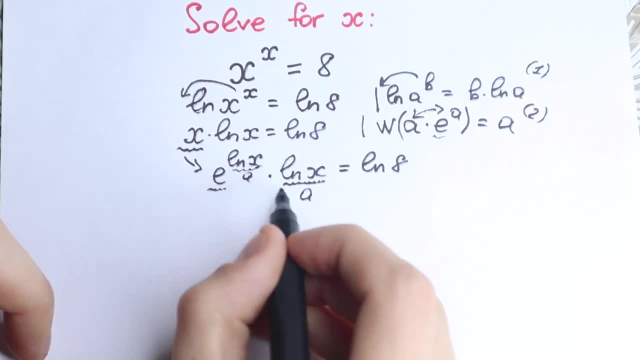 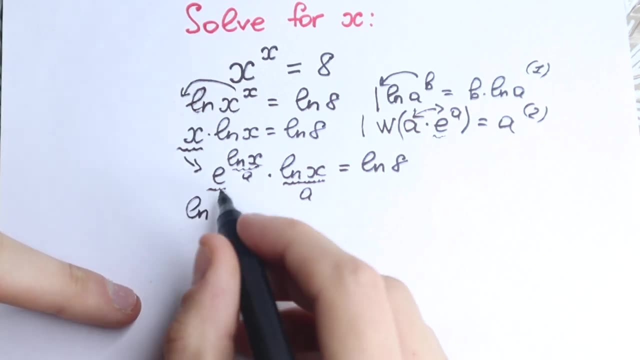 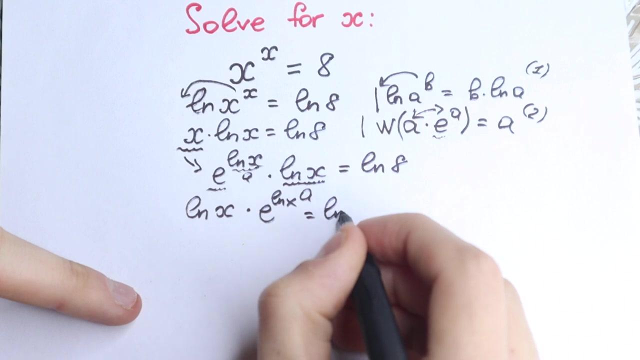 same nature log x. so we have e to the power a times a. so this is like completely the same as right here and i. i wanted to change an order for you. so we have natural log x times e to the power. natural log x equal to nature. natural log 8. okay, i change in order. we can do this because we have 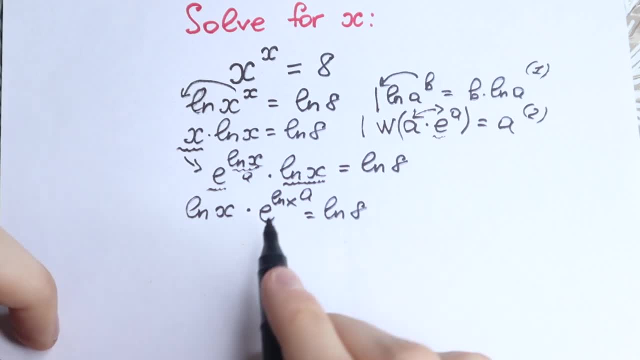 because we have multiplication right here, so we can easily change an order with this one, with this one and this one. so right now, let's look closely to this. so right here we have natural log x. as i, as i told before, this is our a in our 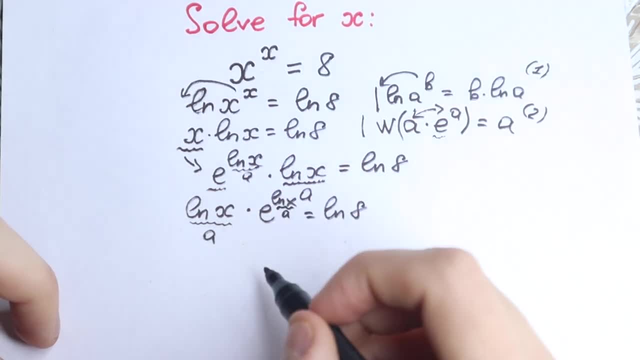 head and we have the same a as right here, so this is our a as well. yeah, so we have a times e to the power, a equal to natural. okay, we don't need this right now. we need this expression because right here we can easily apply lambert w function from this all expression, and we need to do this on the 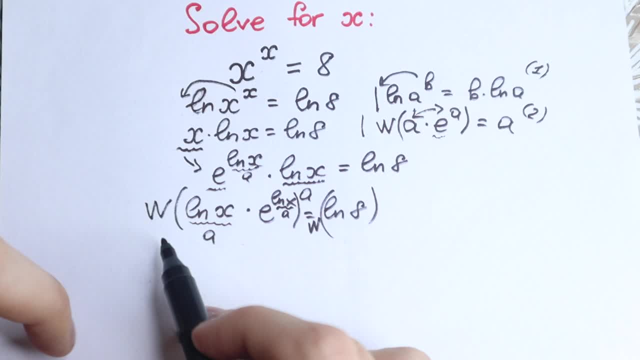 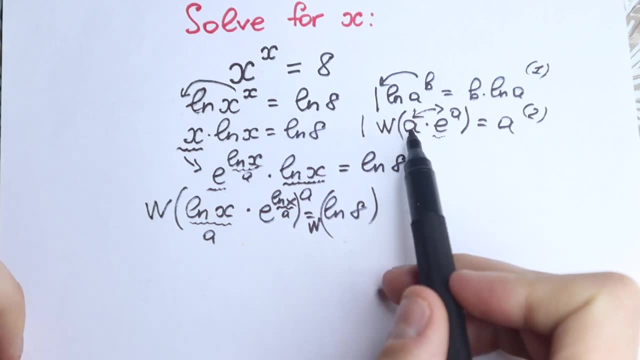 on the right hand side, on both side. if you do something like this, you can easily apply this on the left hand side. you need to do absolutely the same thing with this nature: locate right now. let's look closely to this rule. so we have a times e to the power, a okay, and right here we have this. 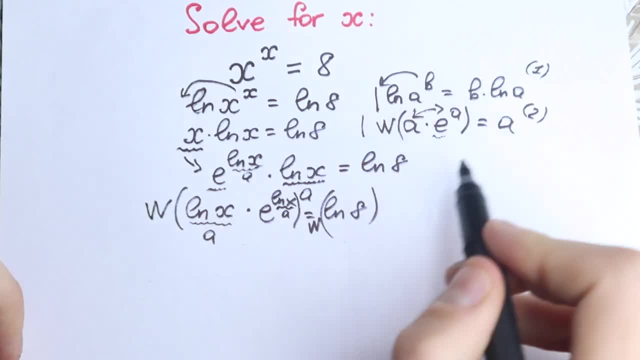 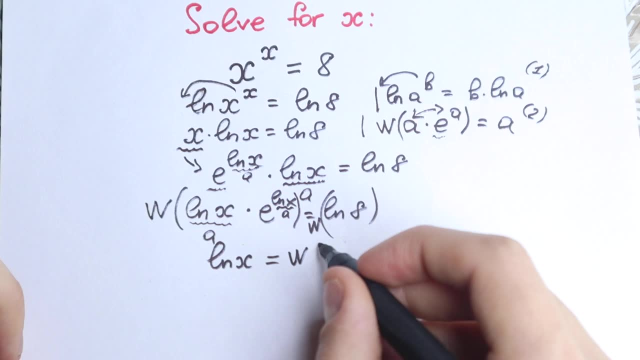 expression. but instead of a we have nature log x. so this is our answer to this left hand side. so nature log x, equal to the lambert w function, to the power- uh, not to the power of nature log. nature log eight. okay, really great, this is a constant, because nature log is a. 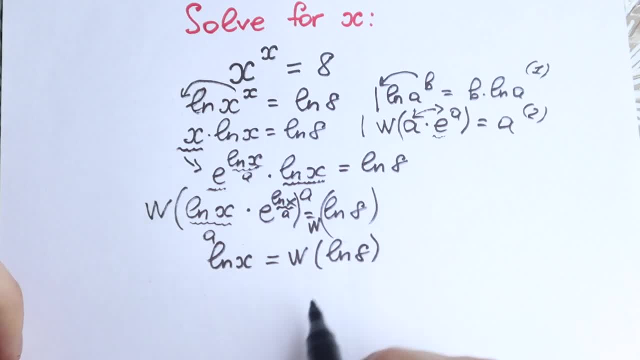 constant and lambert w function in this point. this is a constant, yeah, and nature log x. this is our variable. from here we can easily find our x. we don't have any power, so it's it's really great, but for this question i suggest you to learn this trick. so i just create base, base of e on both sides. 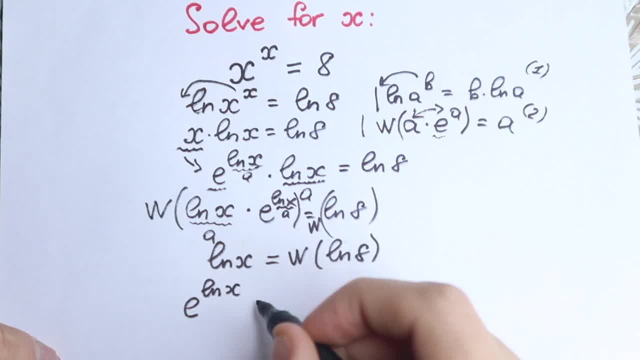 so we have base of e of nature log x equal to base of e of lambert w function nature log, nature log 8.. okay, i just changed nothing. i just created base of e on both sides. i just applied this base of e on both sides and i write right. 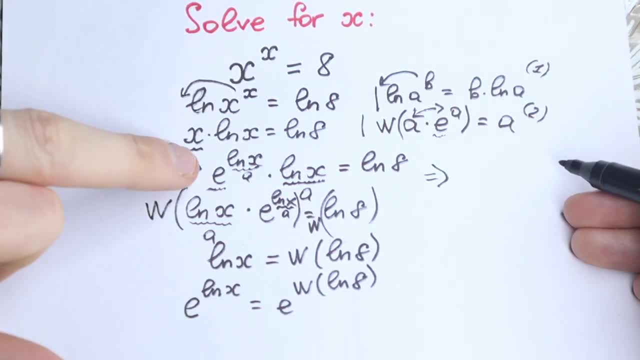 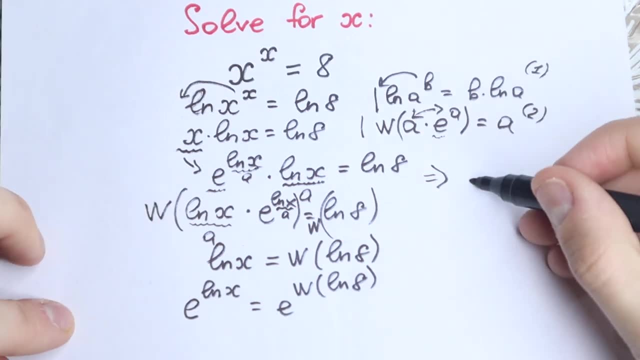 here on the top. so e to the power nature log x. let's go back e to the power nature log x. this is the same as x. okay, we can easily change this. we can easily write it as x, x equal to, and right here, e to the power lambert, w function of nature log, nature log 8.. okay, this is a constant. e is a. 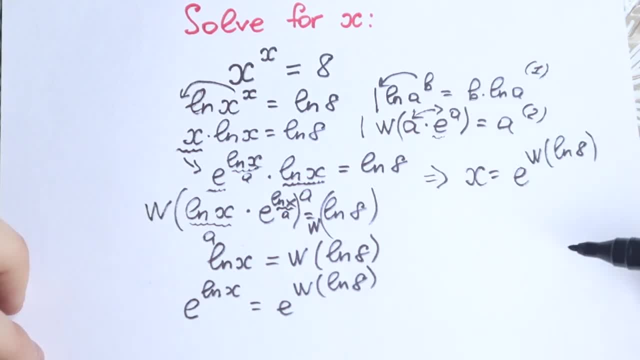 constant, so we can easily find this. but if you solve this question, like on your exam, this is your final answer because you don't allow like to calculate it, to find it exact value of this question, this approximate to this, to this x, to this e, to the power lambert w.